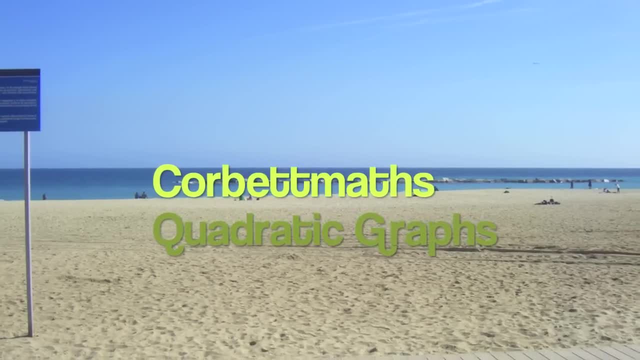 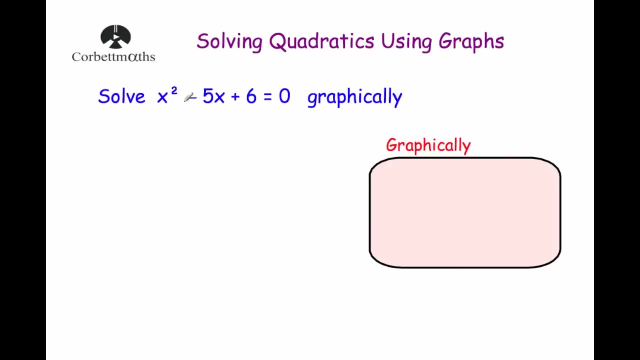 In this video we're going to look at how to solve quadratics by using graphs. So here we've got an example. It says: solve x squared minus 5x plus 6 equals 0 graphically. So, first of all, what we're? 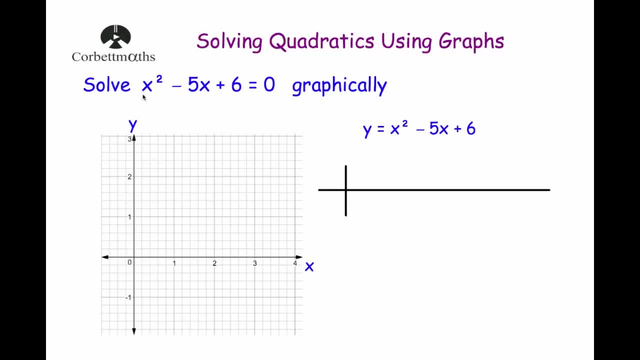 actually going to do is we're going to draw the graph. So obviously the question says x squared minus 5x plus 6 equals 0.. We're actually going to draw the graph, for y equals x squared minus 5x plus 6.. Okay, so I'm going to use an xy table. so x and y. I'm going to choose values of x of 0,, 1,. 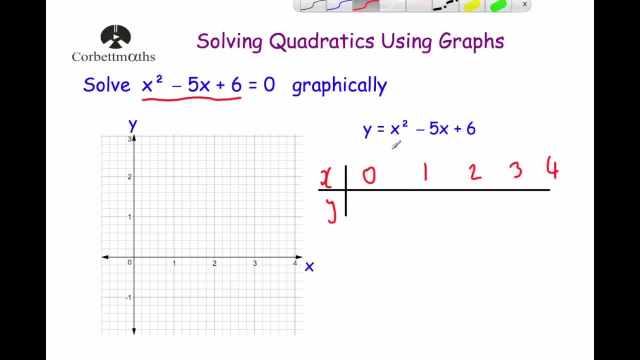 2, 3 and 4, and I'm going to work out what the y value is. So I'm going to square it. so 0 squared is 0 minus 5 times 0, or 5 times 0 is 0. So we've got 0 minus 0 and then plus 6.. So whenever x. 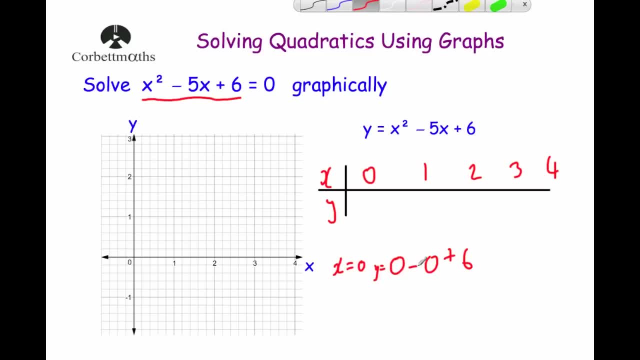 equals 0, y equals 0 minus 0 plus 6, which equals 6.. So that's our first coordinate: 0, 6.. So 0, 6. it's actually way up here. Okay, next one: 1.. So 1. 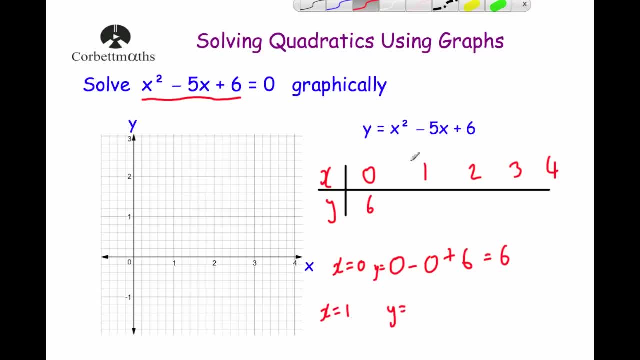 squared is whenever x is equal to 1.. y equals 1 squared, which is 1 minus 5 times 1.. That's minus 5 plus 6.. 1. take away 5 is minus 4 plus 6 is equal to 2.. So that's the other coordinate: 1, 2.. So 1,. 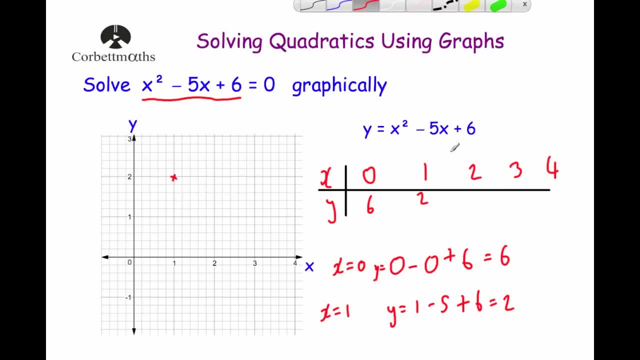 2.. Great, we can plot that one on the graph 2.. Well, 2 squared is 4.. x equals 2.. y equals 2 squared is 4 minus 5 times 2 is minus 10 plus 6.. 4 minus 10 is minus 6 plus 6 is equal. 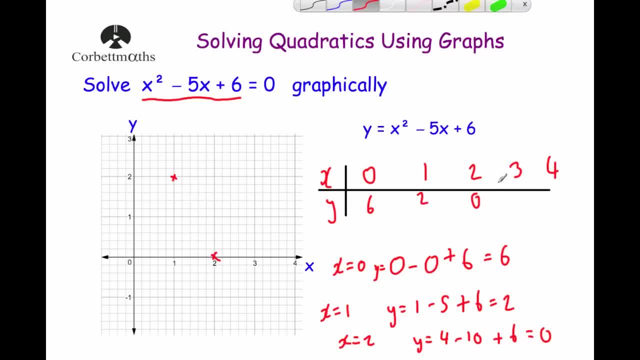 to 0.. So that's 2, 0.. That's our next coordinate, 3.. So whenever x is equal to 3, y would be equal to Well, 3 squared is 9 minus 5 times 3 is 15 plus 6.. y equals 9.. Take away. 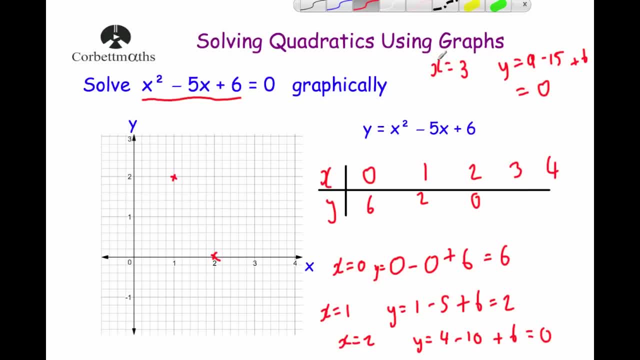 10 is minus 6 plus 6 is 0.. So our next corner would be 3, 0.. So that's the coordinate there. And finally, 4 whenever x is equal to 4.. Need a bit more room. x equals 4.. y equals 4. squared is: 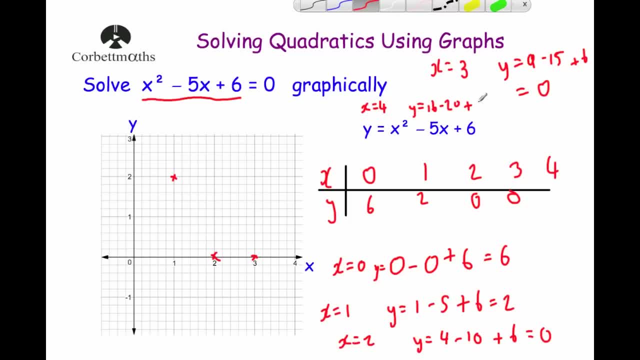 16 minus 20 plus 6.. That's going to be equal to 2.. So that's our last coordinate: 4, 2.. And then we would draw the graph of the curve through that. So here's the graph of y equals x squared minus 5. 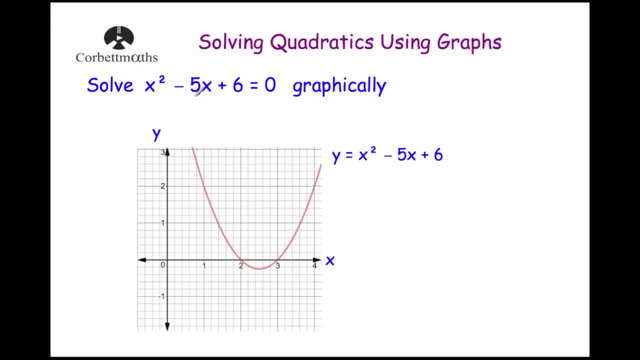 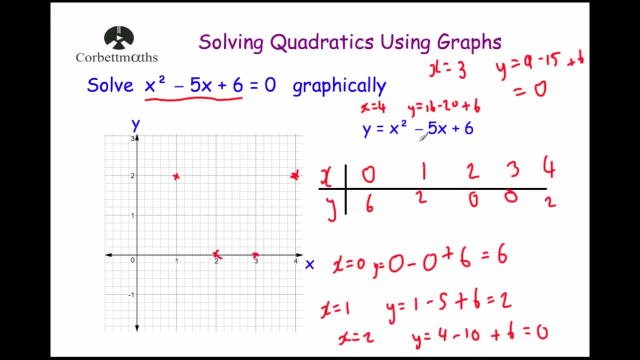 6. Now, remember we're trying to find whenever x squared minus 5x plus 6 equals 0.. Now from our table we can see that happened on two occasions. When x was 2, we got x squared minus 5x plus 6 to. 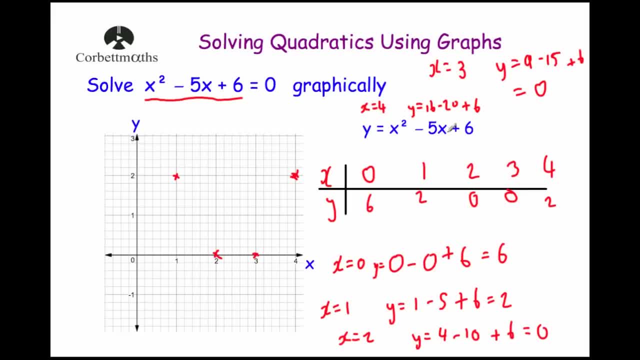 be 0, and whenever x was 3, we got x squared minus 5x plus 6 to be 0. So our answers are: x equals 2 and x equals 3.. Now I've chosen this example on purpose, because I knew that it had integer whole. 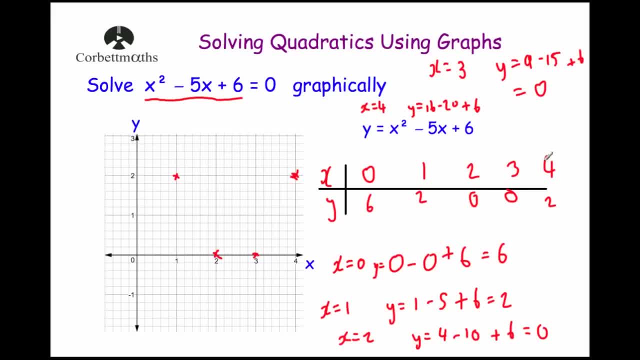 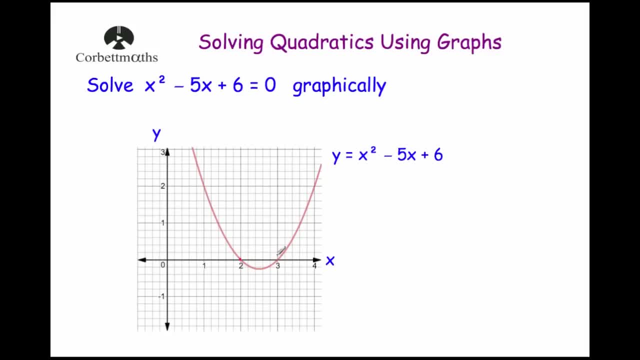 number solutions, and I knew it was going to be 2 and 3.. Now, if we go back to the graph here, we're trying to find our solutions. Now the other solutions are whenever x equals 2 and x equals 3.. Now, the good thing about a graph is it tells you or shows you every single. 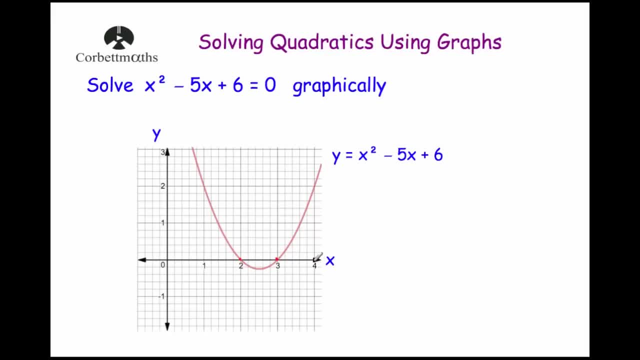 output for your inputs. In other words, whenever we have x and we put in various values of x. So whenever we had x was 1, we know that y would be equal to 2.. Whenever we had x is 2, we knew that you know y was going to be. 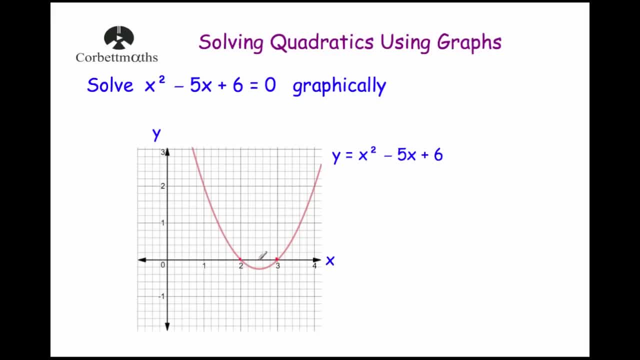 equal to zero. when, if we had x to be equal to 2.5, we know that our y, our output, our answer would be equal to minus 0.22, something like that. now, that's the slight disadvantage with solving um these equations graphically. sometimes, um, whenever you're solving an equation or quadratic. 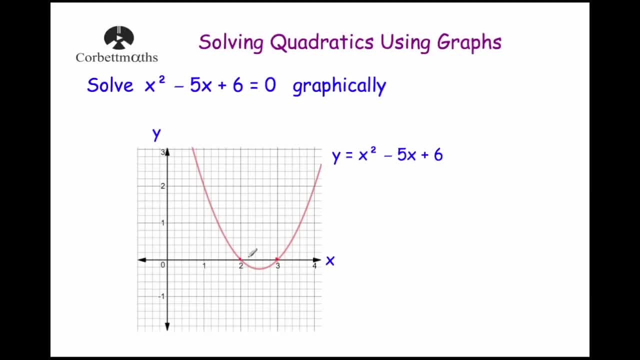 graphically. the solutions might not be whole, it might not be whole numbers. so this was quite a nice one. um, if they're not whole numbers, you're sort of finding approximations or estimates, and there's slightly better techniques to find them. so our solutions were: x equals 2 and x equals 3. 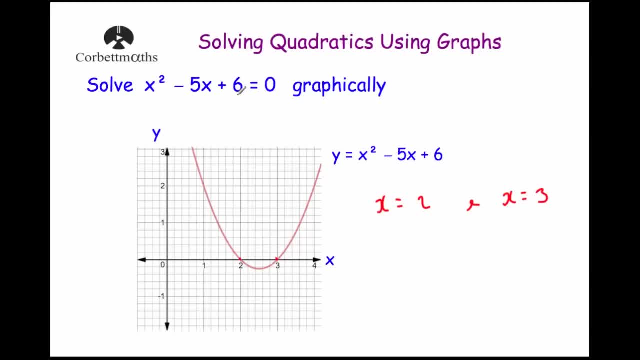 now, if your quadratic equation equals zero, to find the solutions all you need to do is to plot that quadratic graph and you just find where it crosses the x-axis. because if the quadratic equation equals zero, that means that y, or the height, is equal to zero. so you 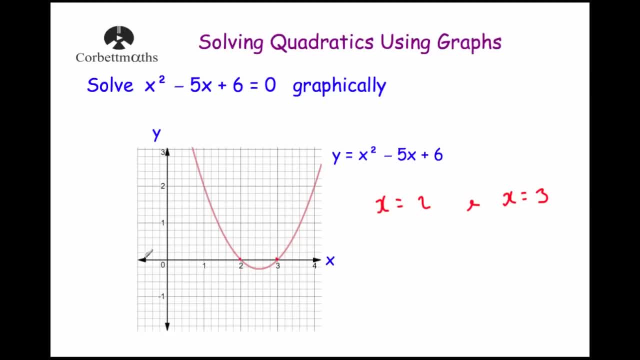 just trying to find out when the height is zero. now, the height is zero, obviously, whenever crosses the x-axis. so that's all you've got to do. if you've got a quadratic and equal zero, you draw the quadratic graph and find where it crosses the x-axis. that might be two different locations, like. 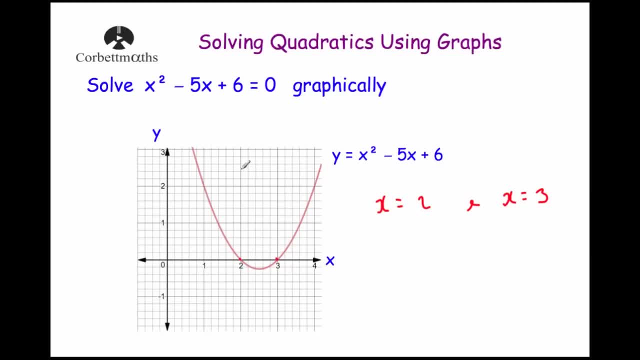 this. it might sometimes just touch it at one location, or sometimes it might not cross it, so that means you couldn't actually solve the equation. but that would be very unlikely to be given to you in an exam. be particularly nasty, okay, so let's have a look at our next. okay, so here's our second. 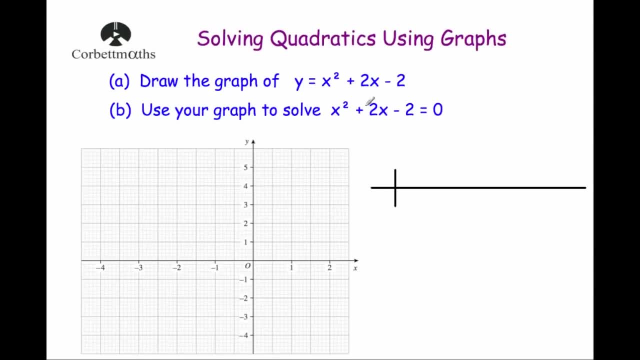 example, part a draw the graph of y equals x squared plus two, x minus two, and part b use your graph to solve the equation x squared plus two, x minus two equals zero, and this is quite common um in the gcse, where you get part a to b draw the graph and part b to be actually use it to get. 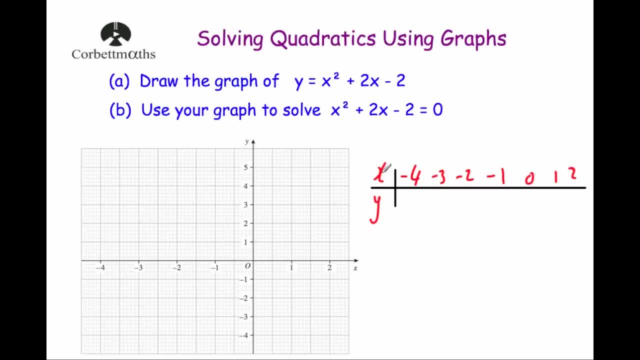 the solutions for whenever it equals zero, and so what we've got is we're going to do an x- y table for part a and we're going to get our values for y. so we've got minus four to two and let's work them out. so we're going to square the numbers, add, double the number and then take away. 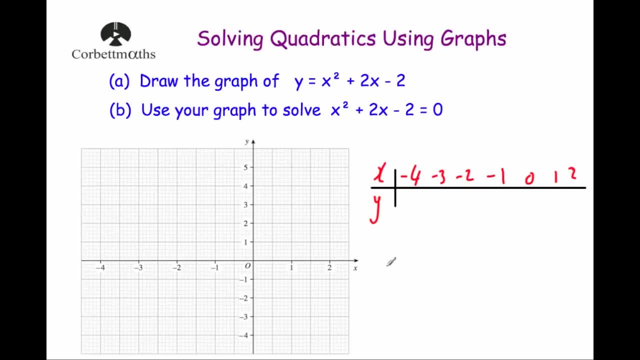 two. so let's start off with minus four. so minus four times minus four is sixteen. uh, double it would be minus eight. so add minus eight. so this means take away eight and then take away number two, and when you- whenever i work that out, or you work that out, you get that to be six. so y would be. 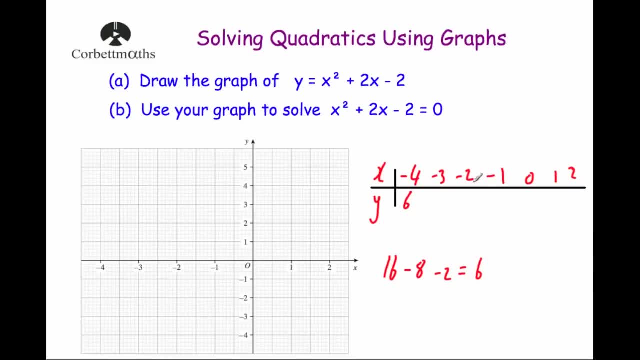 six, and then we just work out all the others using the same technique, and there are one minus two minus three, minus two, one and six. okay, so we've got our points, now we're just going to plot them. so, minus four, six, minus three, one, uh, minus two minus two minus one minus three, zero minus two, one, one. 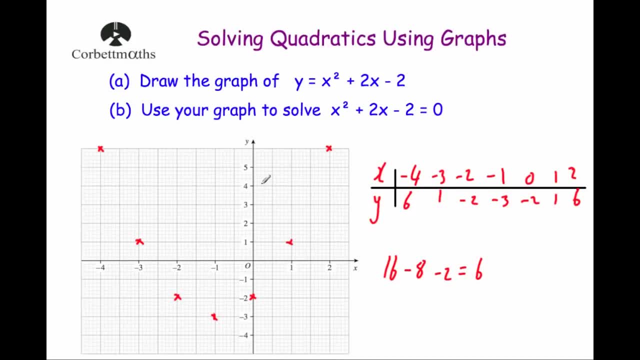 and two, six. now we're going to put a code for them. okay, so we've got the graph. um, i've seen better graphs, but it'll do um. so part b: use your graph to solve x squared plus two. x minus two equals zero. so, as you can see, the graph uh is x squared plus two, x minus two, and the equation is x squared plus. 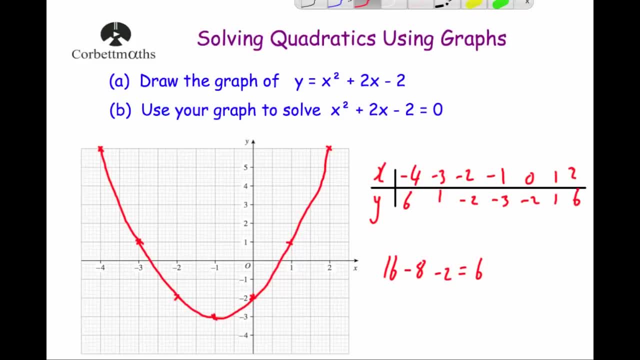 two x minus two, and it equals zero. in other words, we're trying to find where it crosses the x-axis. so, um, it crosses the x-axis here and here. so this solution here would be: um, x equals 0.7, or x equals the resolution minus 2.7, and that's it. so if you were to put 0.7 into this um, into this expression, x squared plus. 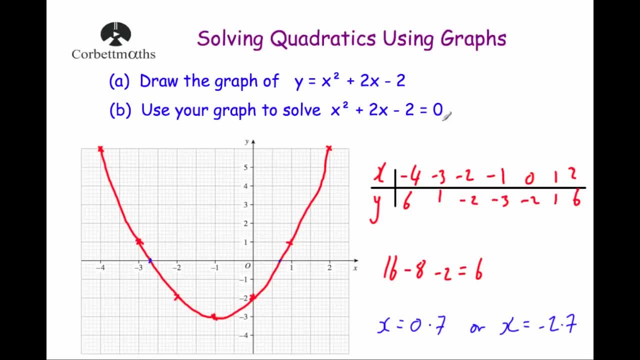 2x minus 2 and you should get an answer close to 0.. now, it's not going to be very, very, very close. it's not going to be perfect because, as i said, this is um, i've drawn the graph, it's, it's not. you know, it's it's. it's not as accurate using the quadratic. 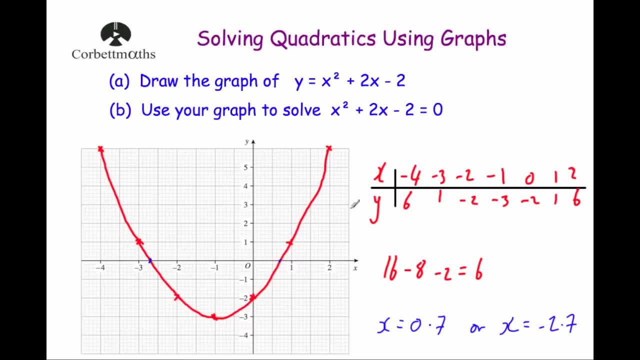 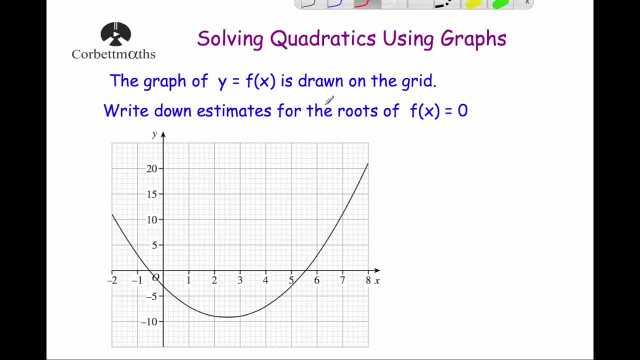 formula completing the square. but it's, you know, it can be asked in the exam. okay, part b. uh, we've done that. okay, next example. okay, next example. i've changed the wording slightly in this question. it says the graph of y equals f of x. so this is the graph: y equals f of x. we don't even know. 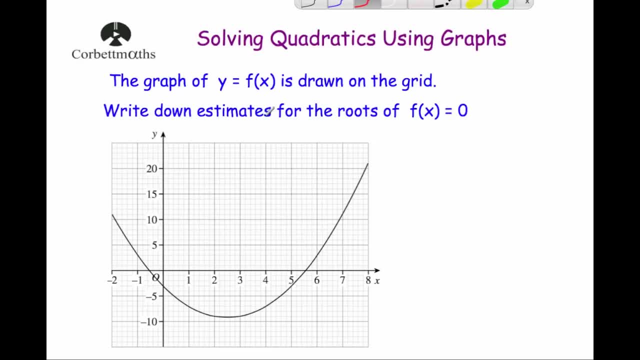 the equation of it is drawn on the grid. write down estimates. for the roots of f of x equals 0.. so roots of x equals 0.. so we're trying to get the answer of f of x equals 0.. so we're trying to get the 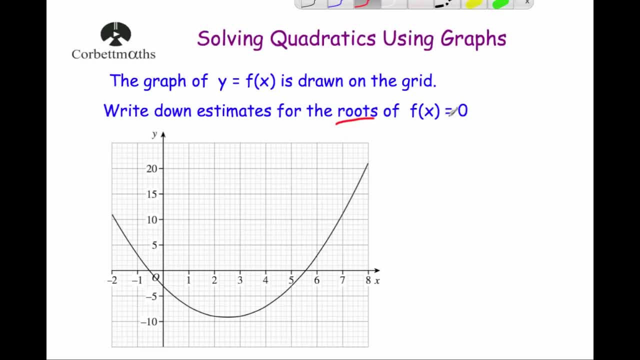 estimates for the answers of f of x equals 0. and again, we've got f of x. we've got f of x. we don't need to know what it is, but we know that equals 0. in other words, we're trying to find when the 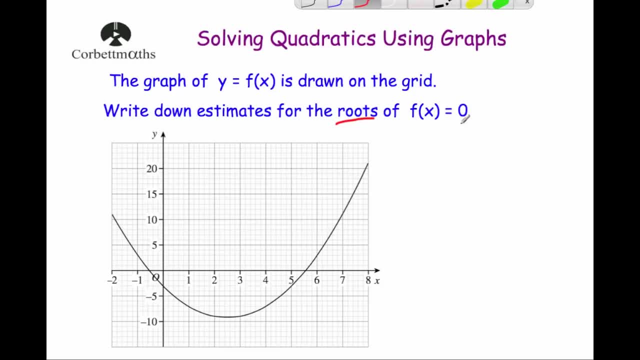 height: 0 y, 0 um, in other words, where it crosses the x-axis. so that's going to be here, and it's going to be here. so this one is x equals 5.6, or the other one x equals minus 0.6 and that's it. so sometimes the the question is where to say it differently, but 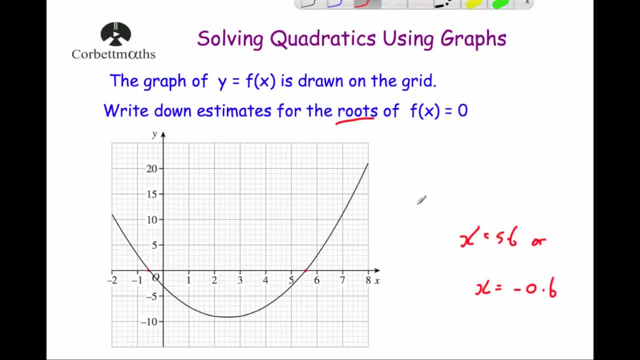 the technique's the same: draw the graph, find where it crosses the x-axis, and that's if the equation equals zero and the graph you've drawn is the same as the expression, the equation on the left-hand side or the bit that's not equal to zero. okay, and the last question. i've changed this one slightly. 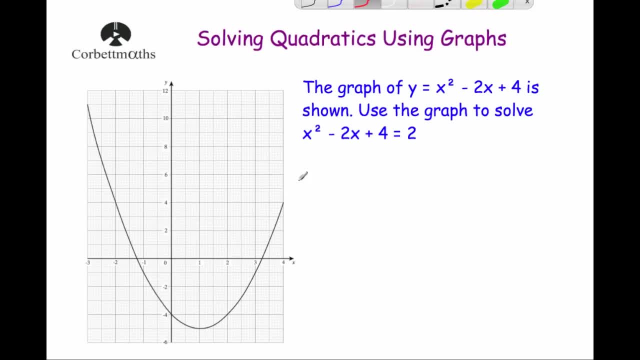 um is what's the difference between x squared minus 2x plus 4 and x squared minus 2x plus 4? so this is the graph: y equals x squared minus 2x plus 4, and we've been asked to use this graph to 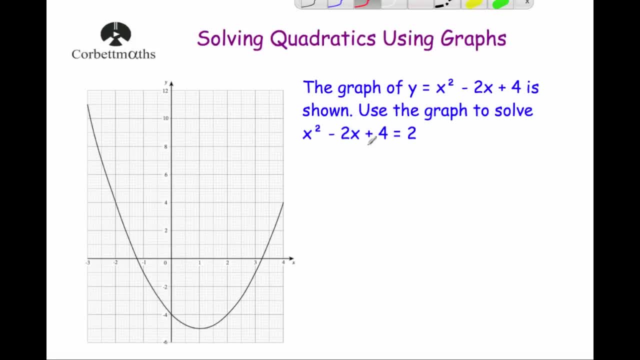 solve whenever x squared minus uh, 2x plus 4 equals 0.. in other words, we're not trying to find this time where it's got a height of 0, we're trying to find when it's got a height of 2. okay, because it's. 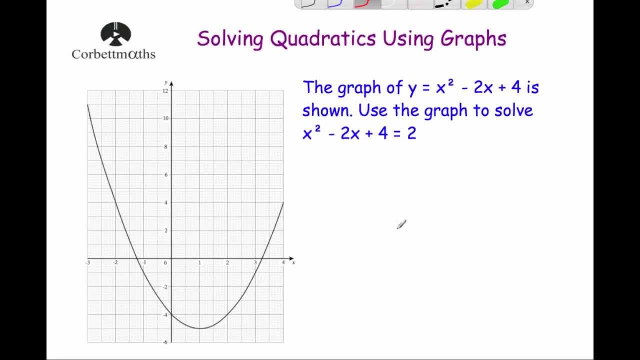 equal to 2 this time. so what we're going to do is um same technique, but, apart from trying to find the one that's well know over here, we're talking about the point that's just at the x-axis, right here, and then we're gonna draw the line here at y equals 2, and reverse when the height is equal to. 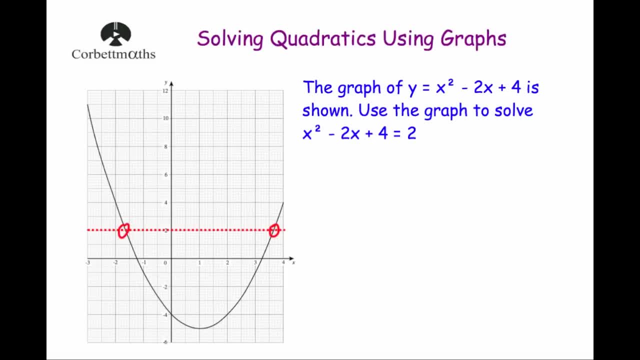 two, and we're going to find where the graph crosses those. okay, so it crosses here at this point here, and it crosses here at this point here. so let's just find what those x values are at those coordinates, at those points. so we'll go straight down there and we're gonna go straight. 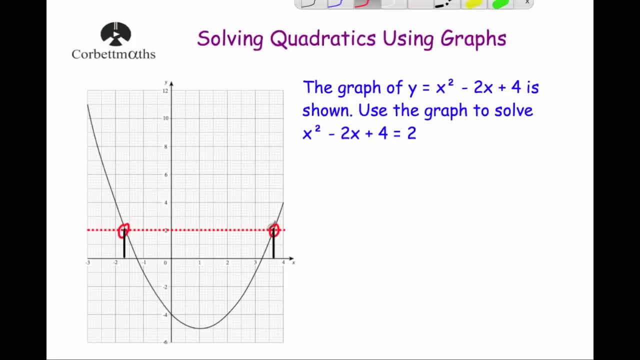 down here, okay, so in other words, put in this value of x. you should get an answer of two whenever you're drawing this graph. okay, and this coordinate here is equal to 3.6, so x equals 3.6, or this one here, x equals minus 1.7. 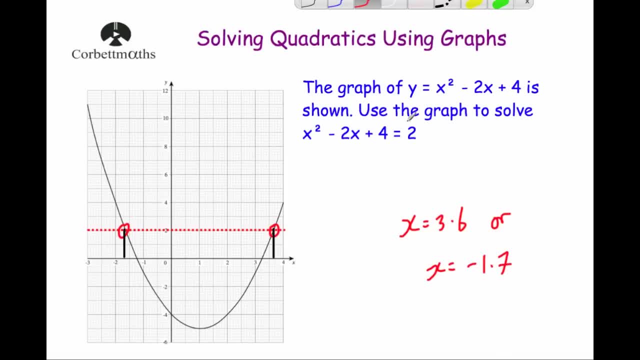 okay. so if the graph doesn't equal zero, okay, and if it equals a different number, what you do is you're just trying to find the x values that give you that height. okay. so what i do is, if it's two, i draw a line. whenever the height is equal to two, or y is equal the graph y equals two, and then i 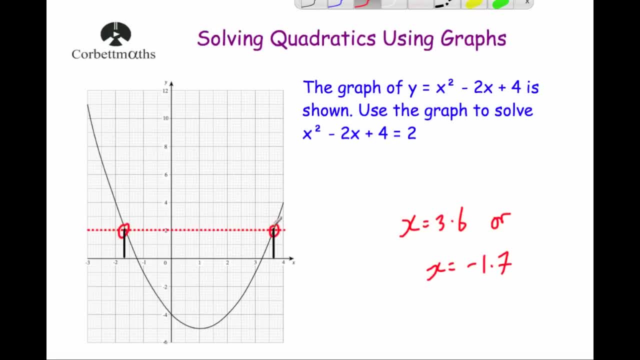 just circle where they cross the curve and then i just find those x values for them. if, for instance, it was whenever equals minus one, say, what i would do is i would draw a line at minus one, which would be here whenever it's got a height of minus one, and then what i would do is find where they cross.